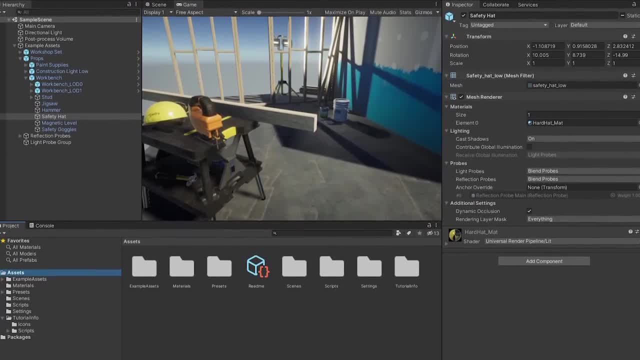 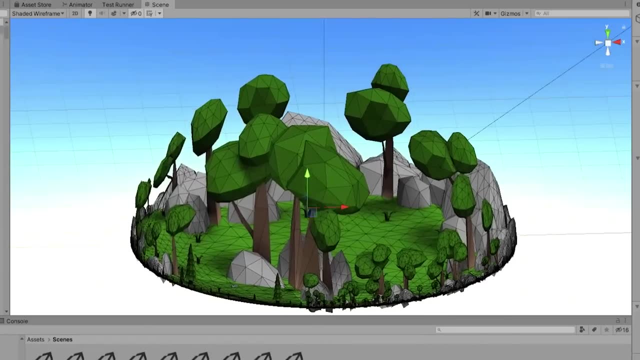 time, and also why I went with Unity as the game engine. There's just more tools and support for it. The first thing I thought about was designing the levels. Building a Hyperbolic editor would take a long time, so instead I decided to use a technique called tile mapping. It's actually really common in games. lots of them use it. Instead, I decided to use a technique called tile mapping. It's actually really common in games. lots of them use it. Instead, I decided to use a technique called tile mapping. It's actually really common in games. lots of them use it. 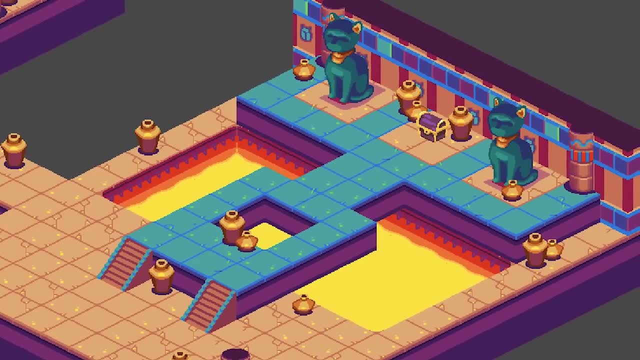 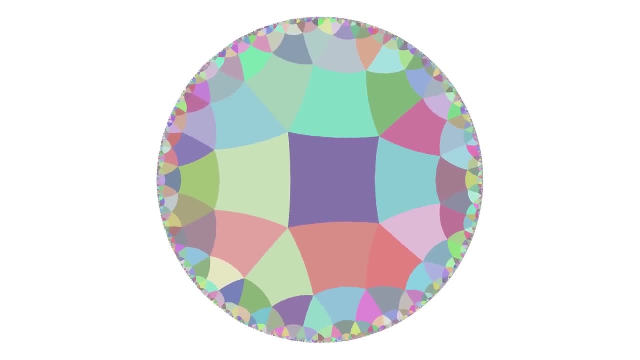 Instead of building one gigantic landscape, you just connect a bunch of smaller tiles together to form it. The only difference in Hyperbolic space is there's a different number of tiles around each corner. To make things even simpler, I only use square tiles and I just change the 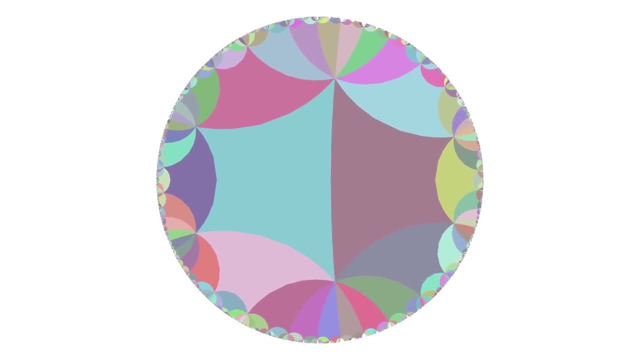 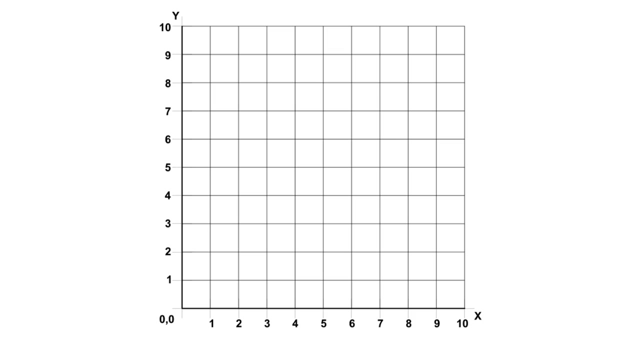 number of squares per vertex to get different curvatures on different levels, including spherical. When it comes to placing those tiles, a grid would be really nice, because I could just place a tile at, say, five comma four and that's it. But you can't. 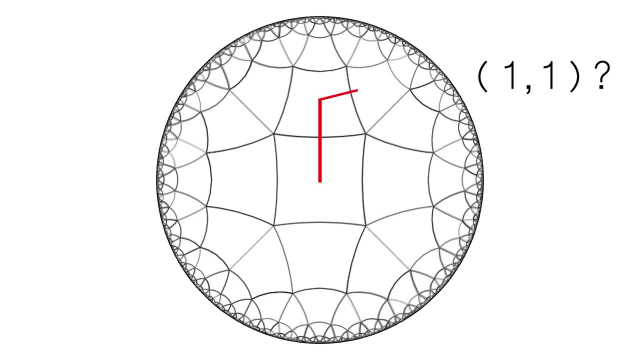 do that with Hyperbolic grids. Remember, up right is a different coordinate than right up. Integer pairs won't work, So I just took the lazy way and just represented tile coordinates as a string of steps from the origin. So this would be the R? U tile and this one the U? R tile. 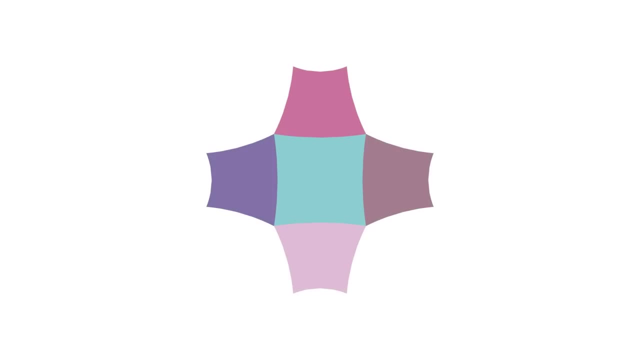 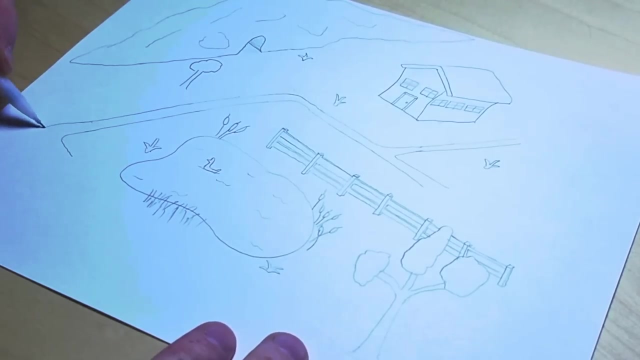 To build the grid, I start at the origin and then recursively expand in all four directions, breadth first. If there's already a tile there, then I just skip it and move on. In Euclidean space it's easy to plan out a level on paper, But I can't do that in Hyperbolic space. 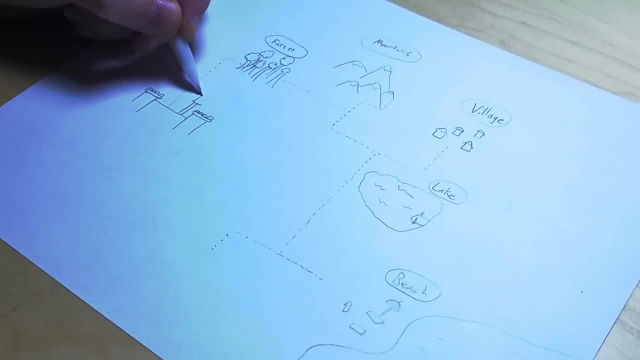 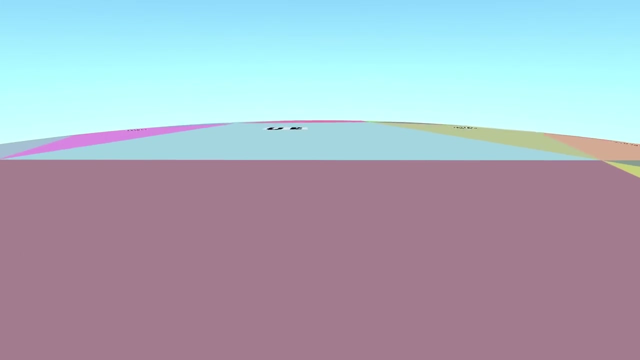 because there's no good way to physically draw it out on flat paper. And, again, I don't want to spend time making a big level editor. so I came up with something easier. Just use the game itself. I just fill the entire level with debug tiles that print their coordinates. walk over to the part of 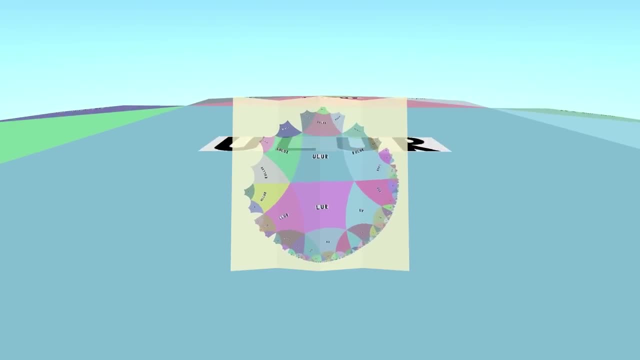 the level I'm working on and then write down which tile goes where and at what orientation. I can preview how that looks, walk over to another section and then just keep doing that. Less important areas can just get filled in procedurally. 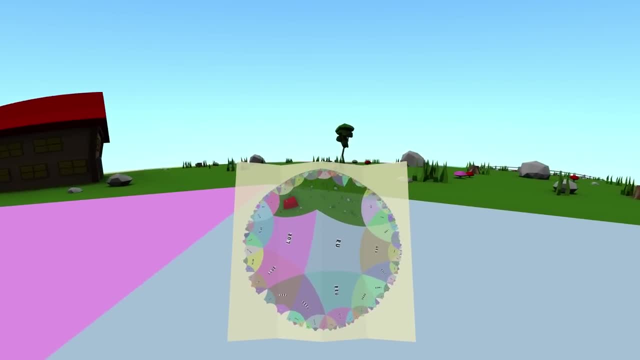 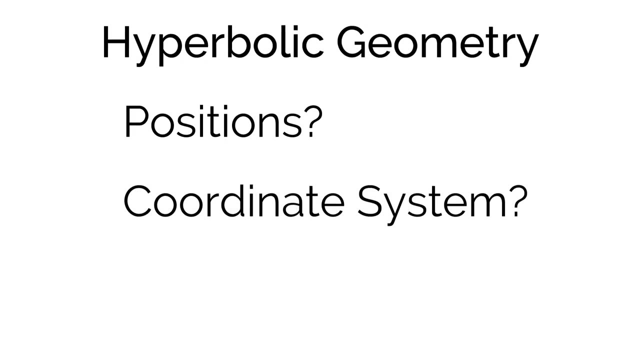 It's not the most efficient, but it was fast enough and worked for me. Now for the big elephant in the room: How do you actually represent a position? What coordinate system can you even use, And how do you transform the tiles or the player, or objects or anything? 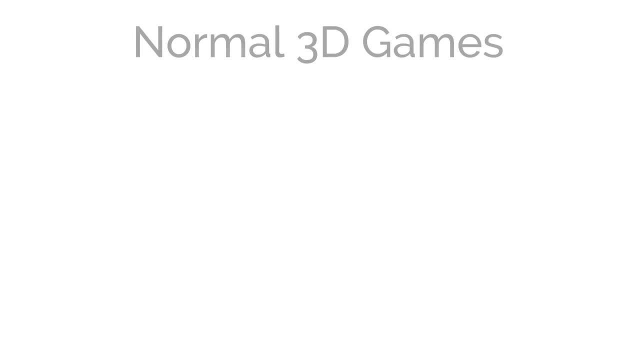 Before I answer that though, here's a quick refresher for how this normally works in 3D games. So there's this concept of a transformation matrix. It's a 4x4 matrix that typically represents an object's rotation, translation and scale. What's really nice about this is you can 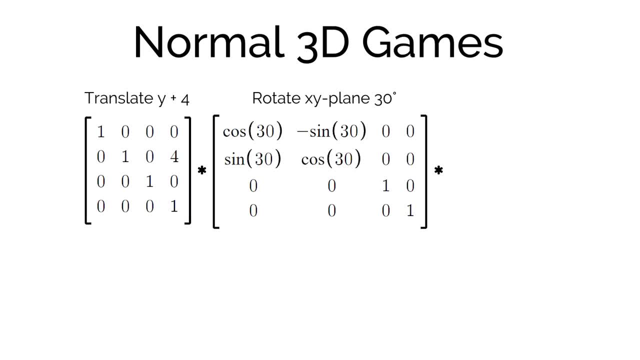 multiply these matrices together to combine a bunch of transformations into just one matrix that gets sent to the GPU. This makes it really efficient and easy to understand conceptually. Well, it turns out that the same abstract concept of a transformation matrix also works in non-Euclidean. 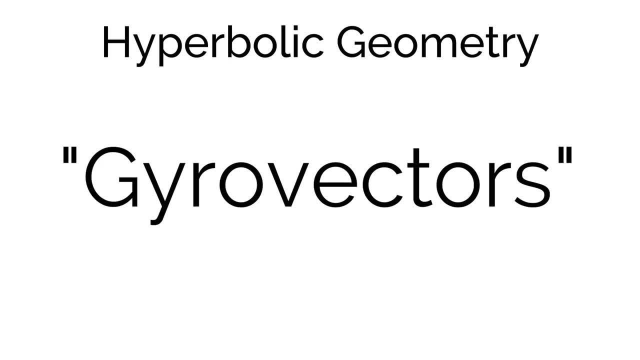 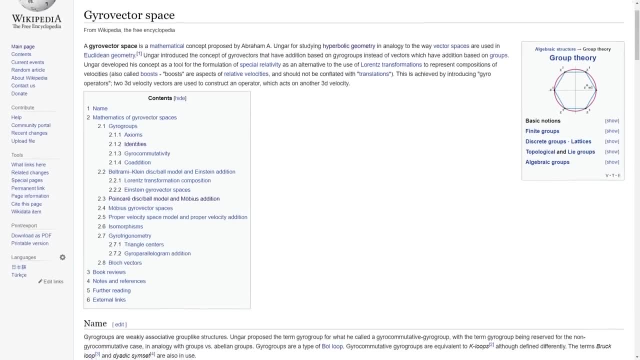 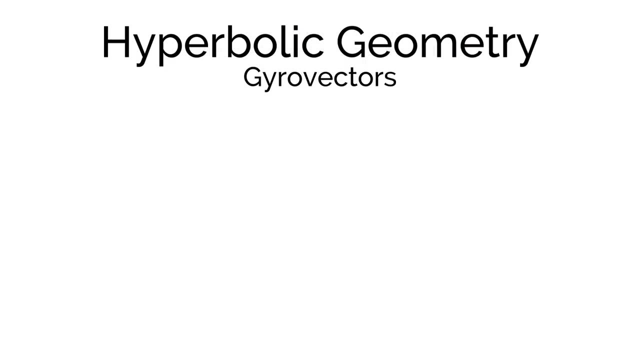 geometry, But with something called gyrovectors. If you've never heard of gyrovectors or gyrovector spaces, you're not alone. They're a really novel concept. I couldn't even find a single YouTube video about it, but they are so useful At a high level. it works exactly the same way. It's a structure that 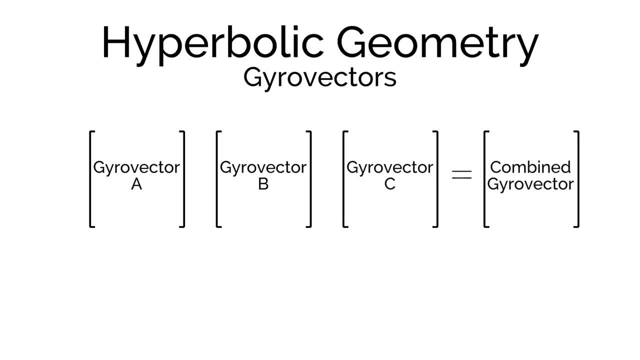 has a rotation and translation. it's just that the multiplication part is a little more complicated than a matrix multiply. Luckily that's all hidden away in the code so you don't even have to worry about those details. Well, sort of It has some different properties, Like normally translations. 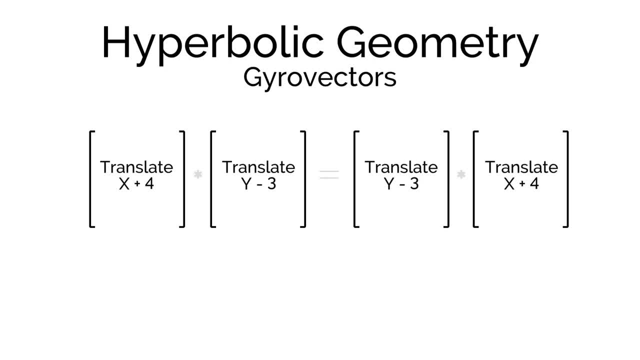 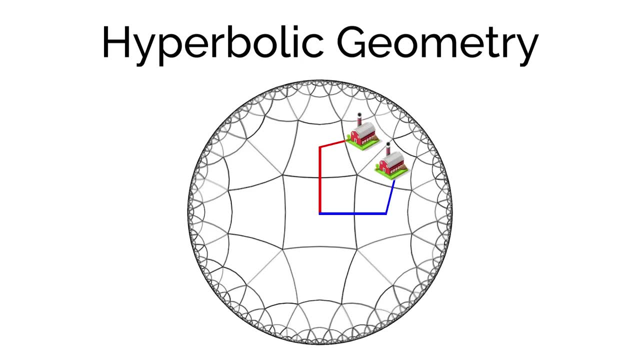 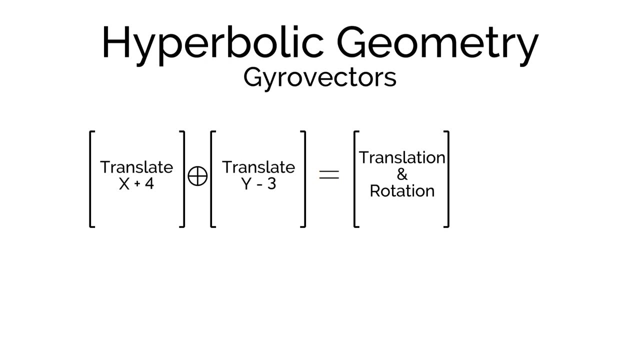 are commutative. It doesn't matter what order you do them in, But gyrovector translations are not. Remember: up right is a different coordinate than right up. Also, the resulting gyrovector can end up with a rotation, even though the ones on the left didn't have any. That's the 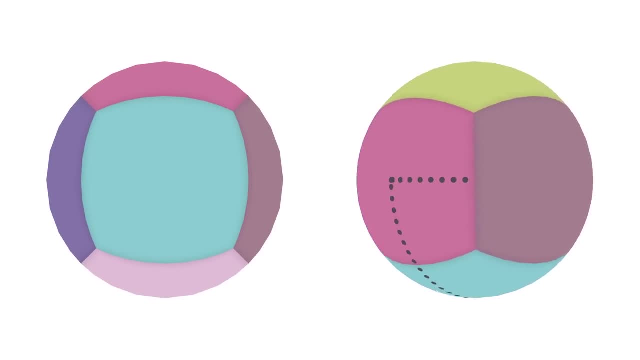 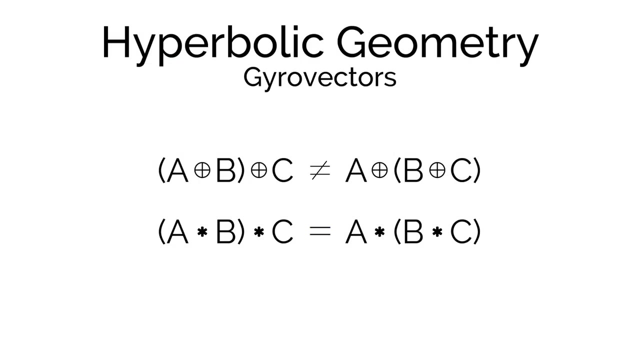 gyro, part of the gyrovector and the result of holonomy, which I talked about in a previous video. Gyrovectors are also non-associative, unlike matrix transforms, which is kind of weird, But we did drop the parallel postulate, so of course we'll have to drop some symmetries. 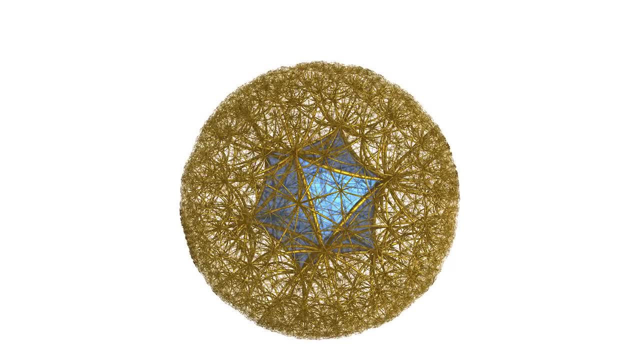 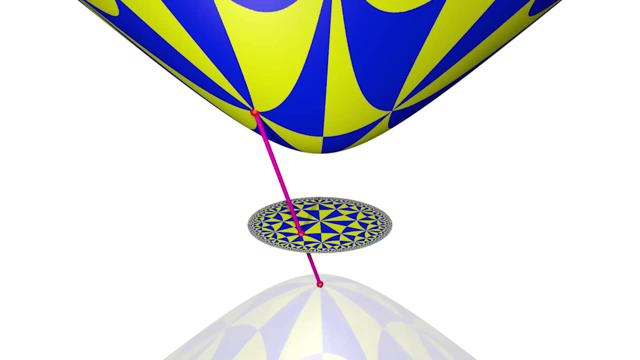 that we take for granted. Anyway, the original paper applied these to points on the Puncari Ball model, the stereographic projection, and so those are the coordinates I use internally. With a few changes, it can also work with hyperboloid coordinates.